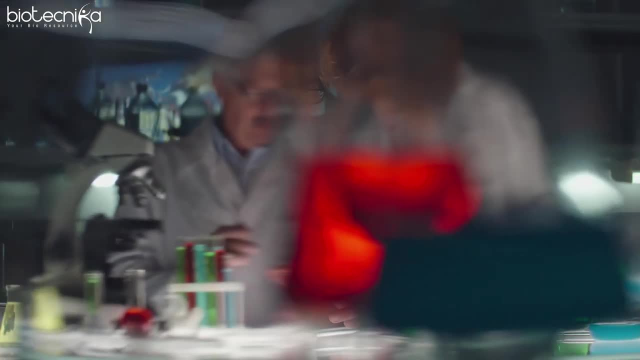 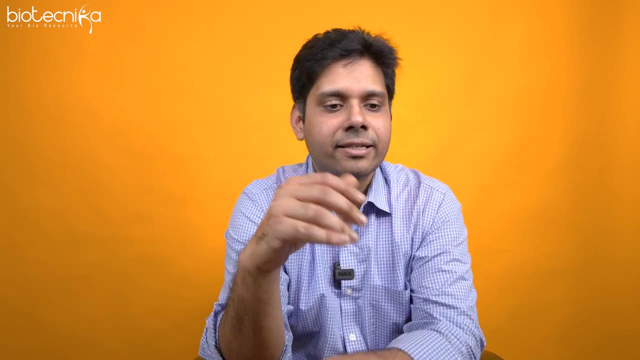 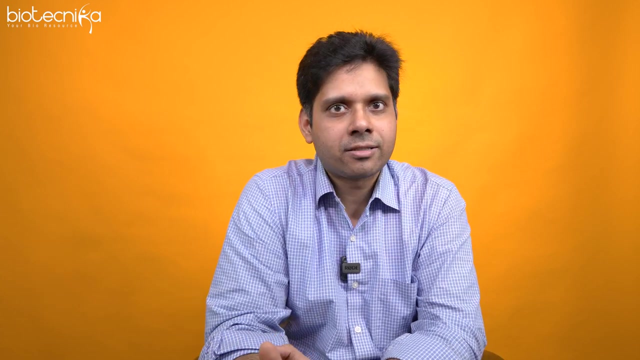 putting in computer and then using statistics to analyze. in computational biology you straight away going from the computer aspect and mathematical models and then you're going to analyze the data. but now let's deep dive and look at what can be the applications of bioinformatics. so the applications of bioinformatics is genomics, proteomics and pharmacogenomics. now genomics is 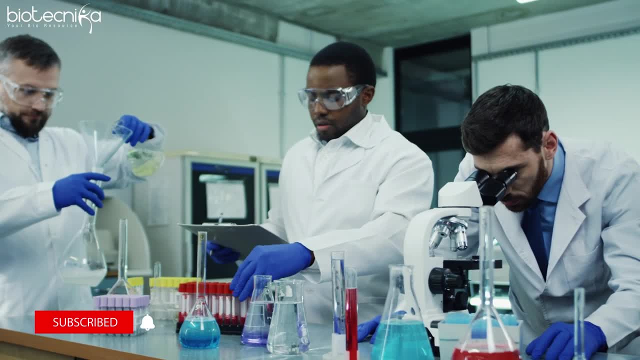 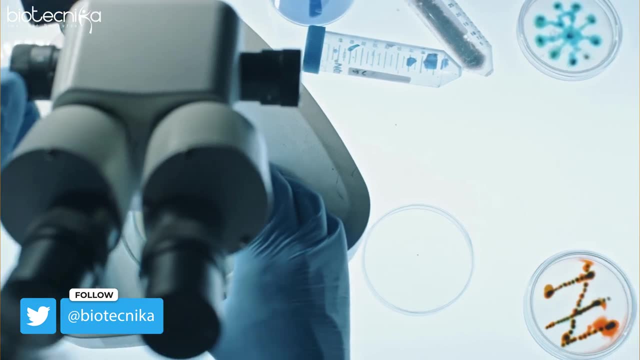 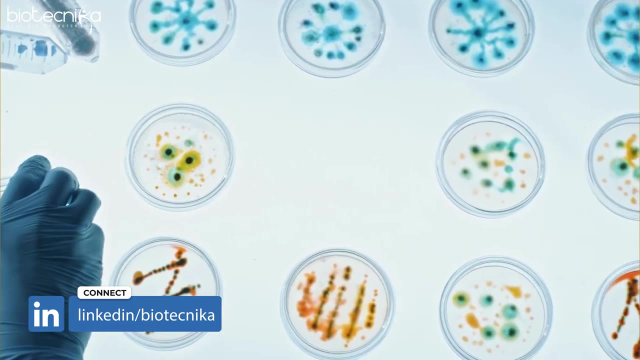 nothing but a sequencing and analysis, analyzing of genomes to understand genetic variations and their implications in diseases. so that's genomics. now, proteomics will be studying the structure, functions and integrations or interactions of protein using computational mod methods, and the pharmacogenomics aspect will be identifying genetic factors that influence a patient's response to. 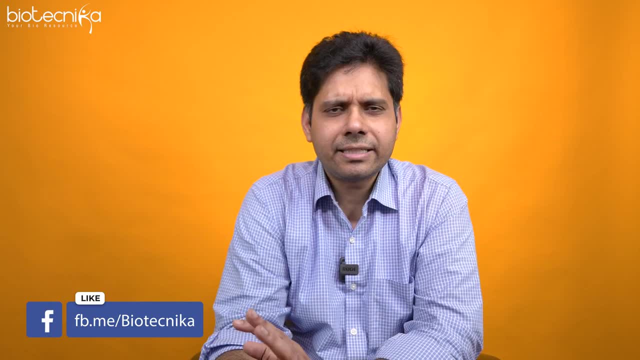 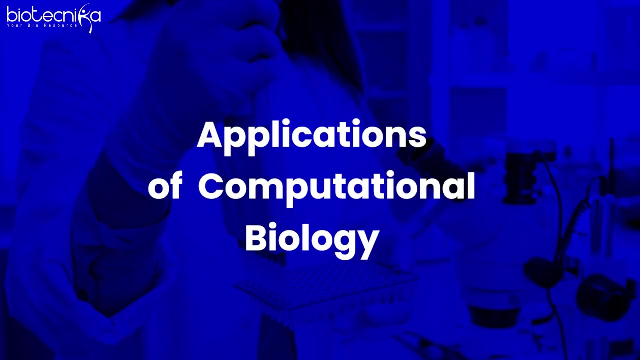 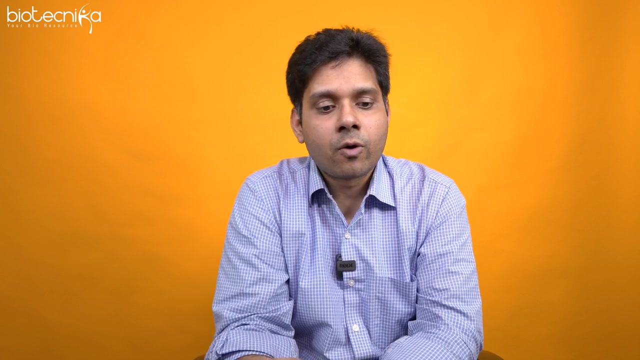 drug help and helping in personalized medicine. now, these are the more or less applications of biologics. but now let us understand what is the application of a computational biologist or biology? now, the first one will be gene regulatory framework or gene regulatory network. so what do we do in this? 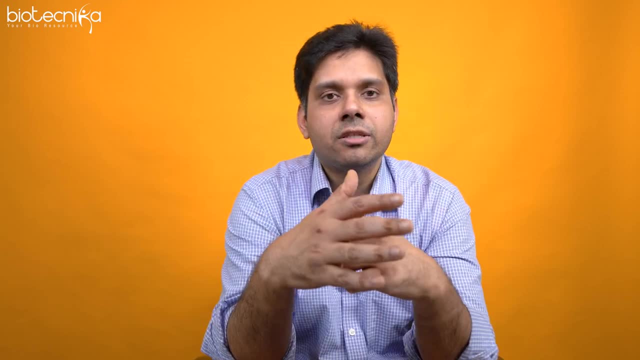 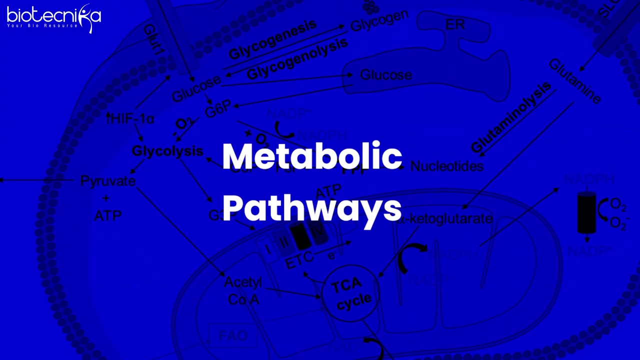 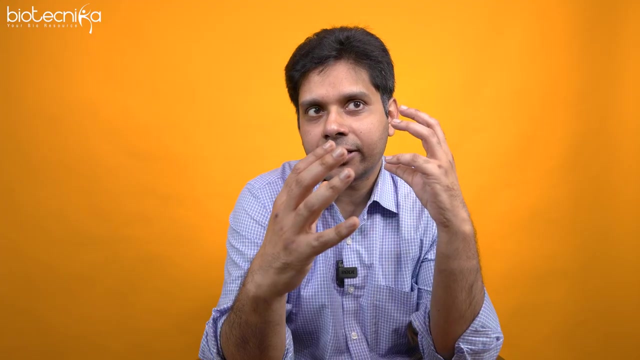 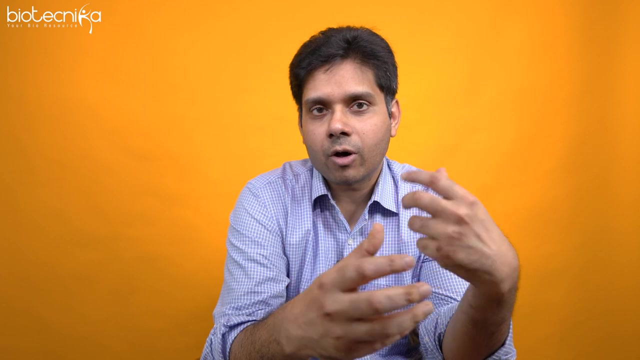 we do the modeling of the interactions between genes to understand how they regulate cellular processes. then the second application will be metabolic pathways. so we simulate biochemical reactions to study this metabolism of cell and organisms. so we are trying to understand how gene is regulating the cellular metabolism. then we are also analyzing how the all the 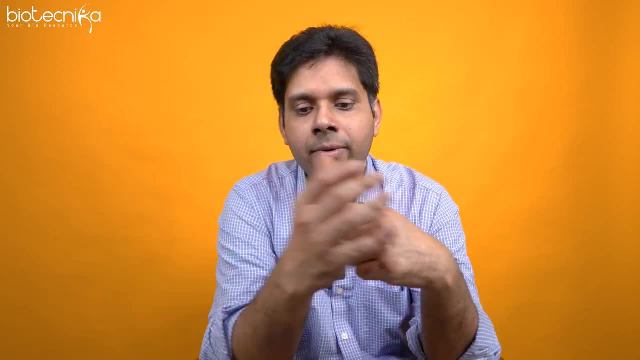 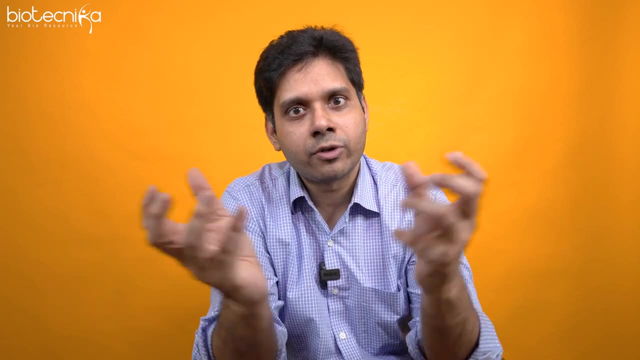 metabolism is happening and we try to simulate that in a virtual environment. and then the third will be protein folding. so we use computational models to understand the 3d structure of protein and how they dock and all that. so that's where the protein folding mechanism we try to understand under this. 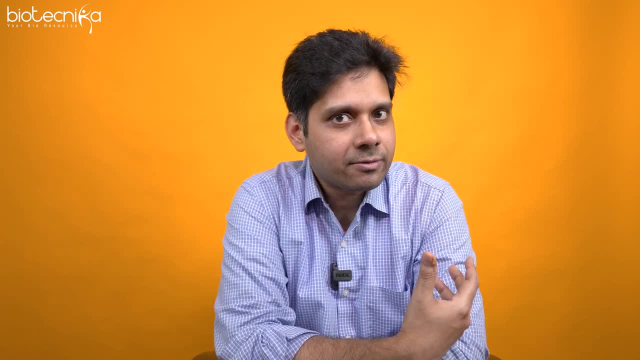 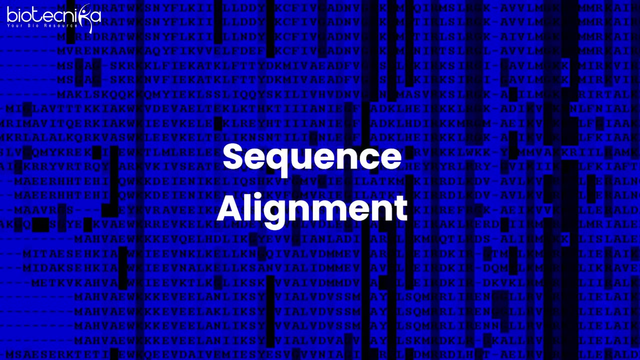 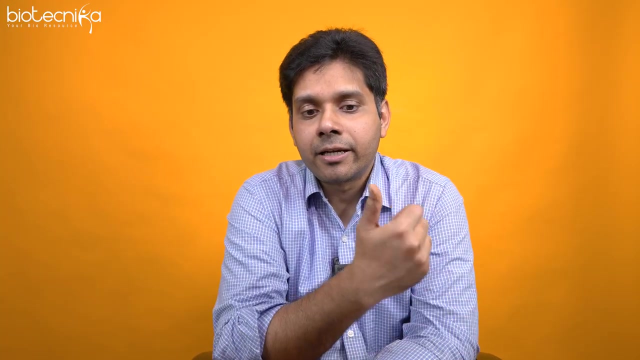 now under in bioinformatics we have various methods which we follow which will be different than the computational biology. so under in bioinformatics we will do sequence alignment, so we will compare the dna or protein sequences to identify similarities and infer the evolutionary relationship. now we will also do structural modeling, so under that we'll predict the 3d structure of proteins similar to 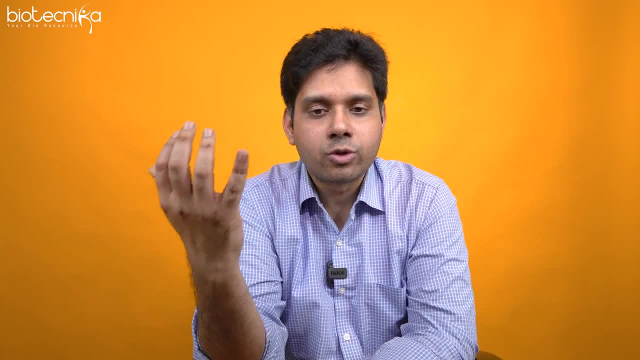 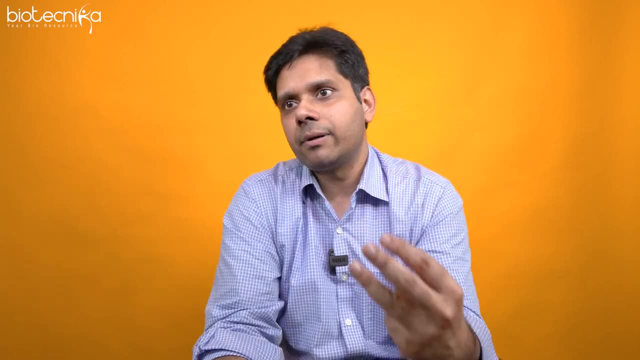 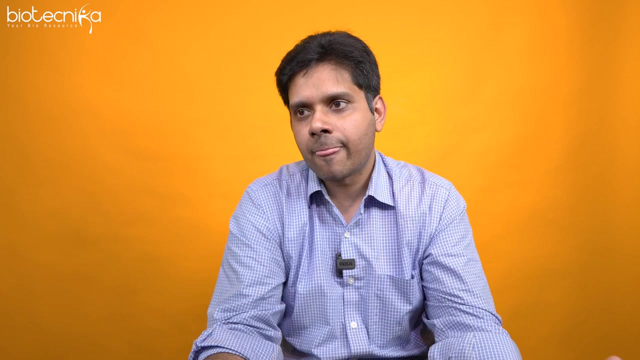 what we do in computational biology, but there we do a 3d modeling using mathematical models. here will be different and we will do the and we will also learn about the amino acid sequences. then the third methods we use is data mining, so we extract meaningful patterns and knowledge from biological data sets. and of course under this comes the machine. 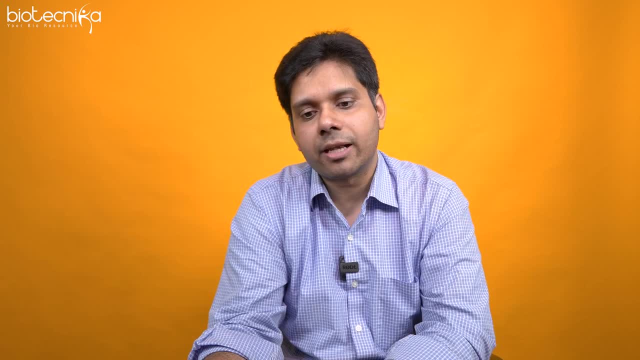 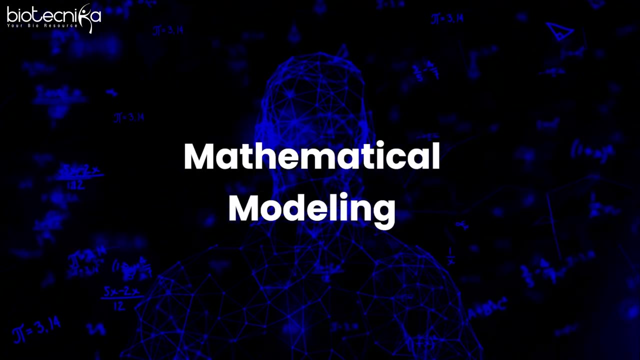 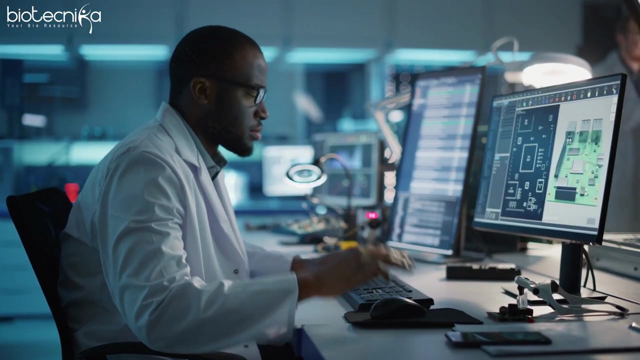 learning, where we use algorithms to develop predictive models of biological phenomena. but now, if we look at the comparison with computational biology, the number one will be mathematical modeling, like i said in the definition itself. so here what we are doing: we are formulating the biological process as a mathematical equation to simulate and predict. 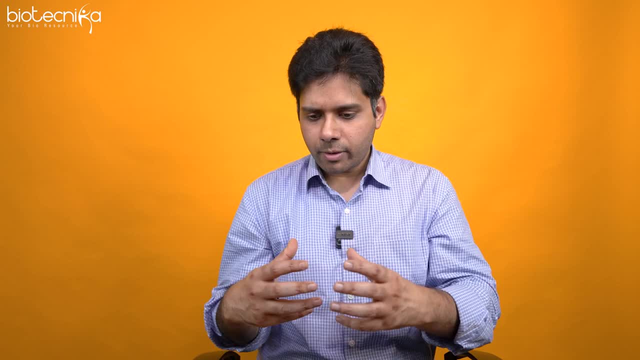 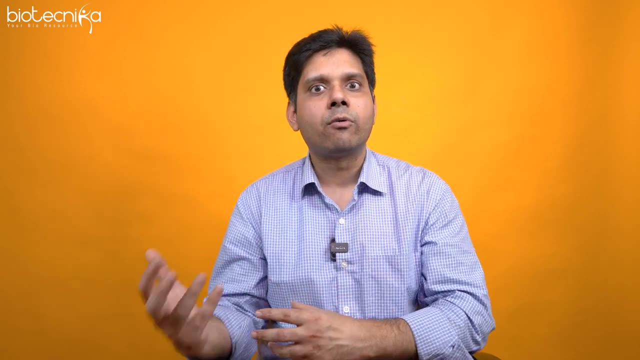 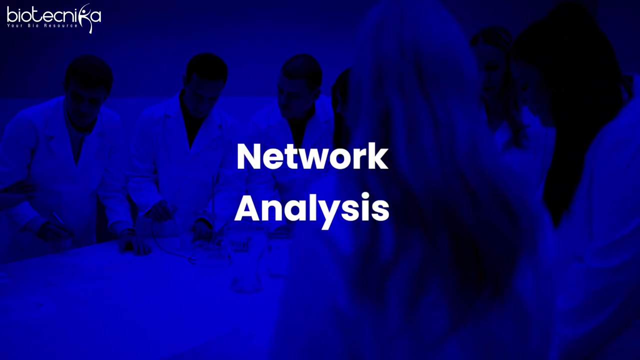 their behavior. so we are taking the biological process and trying to create a mathematical equation and we say, okay, if this happens, that happens. so we try to create an equation, a mathematical equation to predict the next steps. so that's the mathematical modeling we do. the second is network analysis. so we study the biological systems as a network to analyze. 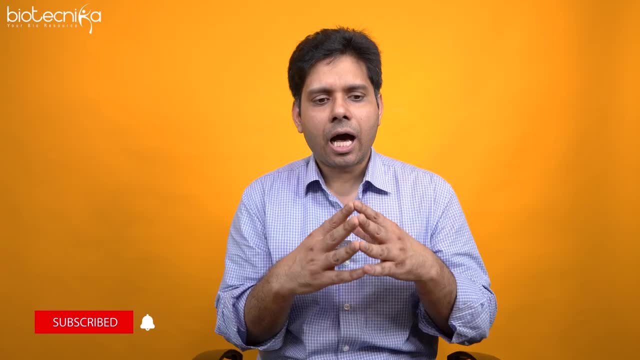 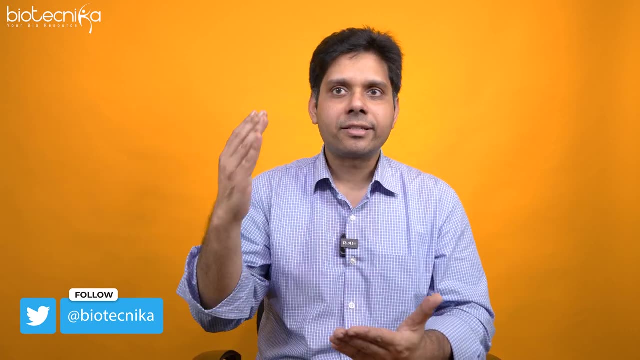 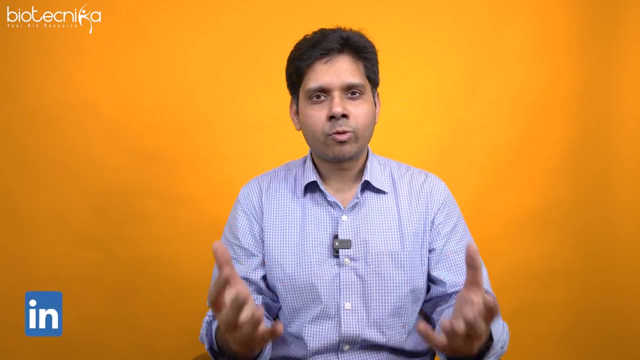 their structure, dynamics and functional properties. so basically, if we see, the entire biological system is not a disconnected system, instead it is a connected system, so it's a kind of a network. so we try to analyze that, to understand the structure, dynamics and functional properties, how it will happen if this happens. that happens, for example, let's say, the the hormonal structure of 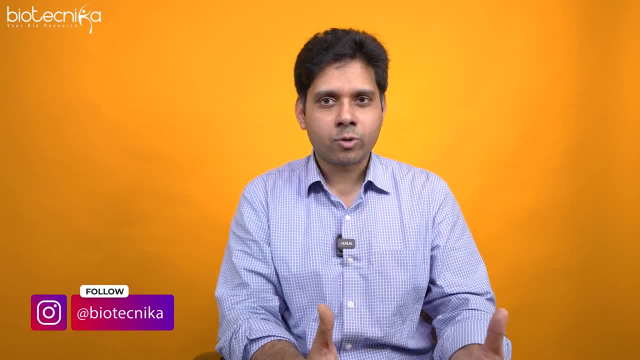 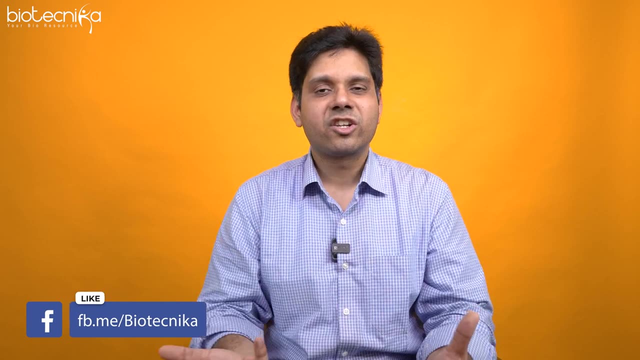 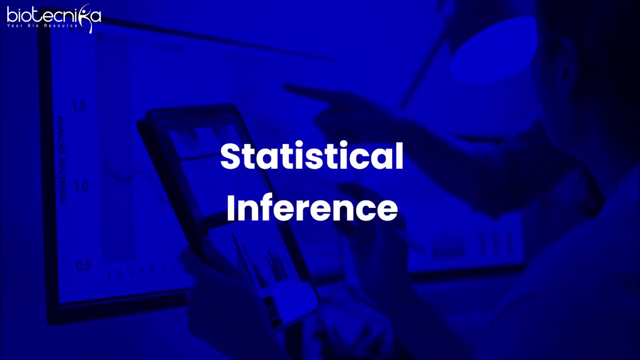 the body. so if, in case, you see the female hormones, like estrogen, progesterone, how they will act and how it will create the, you know more, secretion of a particular hormone. so, understanding all of that and learning that network analysis, that chain analysis we can do, then comes a statistical 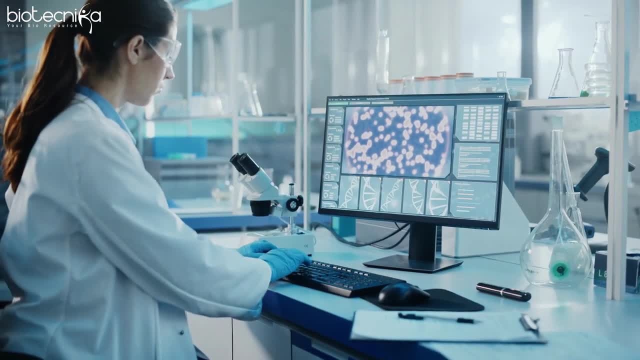 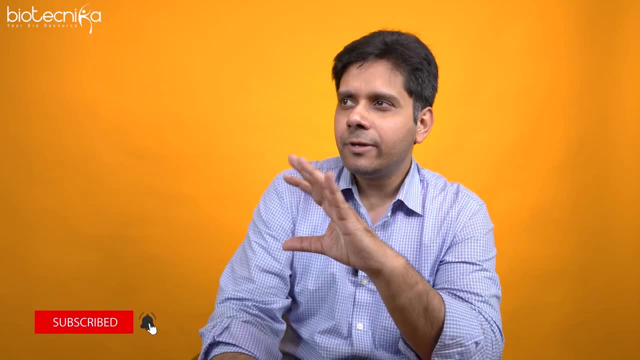 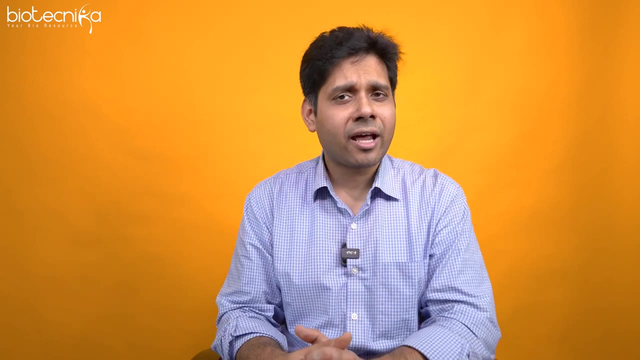 inference. so we use statistical methods to make inferences and draw conclusions from biological data. so this is where these are the methods we follow in computational biology, but we cannot really put both of them apart. like i said, the body is a connected system, the same way all the sciences. 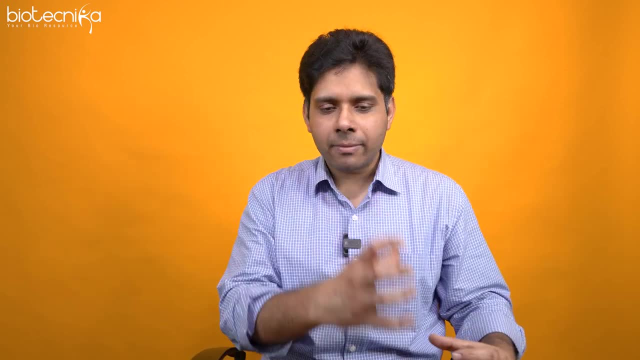 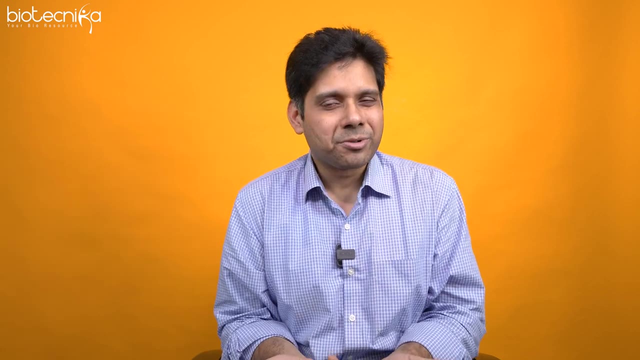 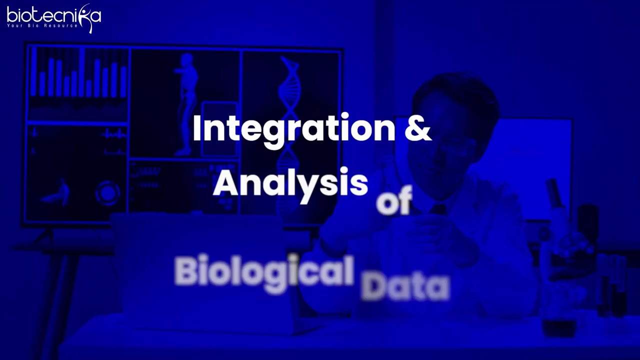 are a connected system. you really cannot remove physics from chemistry. you cannot remove chemistry from biology. you cannot remove biology from bioinformatics. you cannot remove biology from computational biology or computers from computational biology, right? so there has to be overlap. now what is that overlap? the overlap is in bioinformatics. we are. 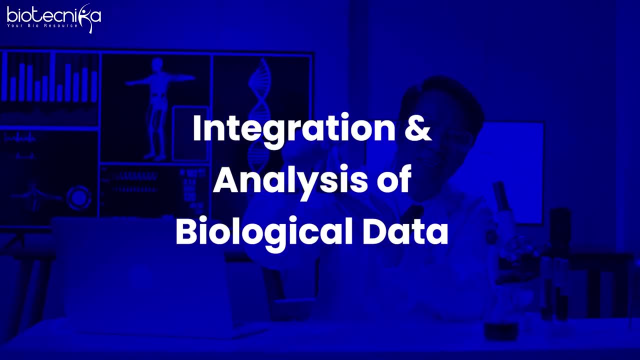 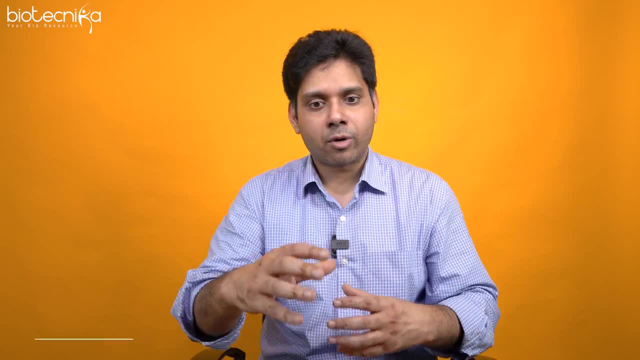 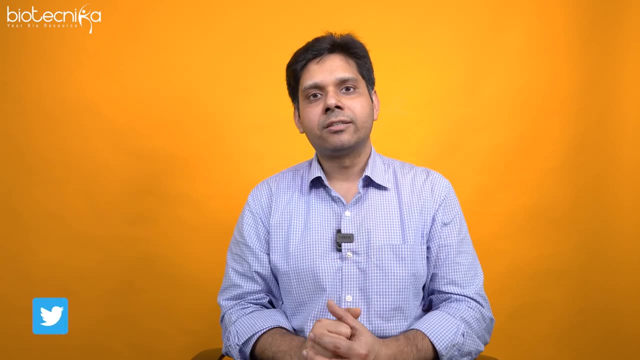 integrating and analyzing biological data and what is happening in computational biology. we are developing applications of computational models. so we are using mathematical models in computational models to predict the next steps, and here we are taking the data from biological side and trying to create the inference. so in both the cases, one is the. we are bioinformatics. 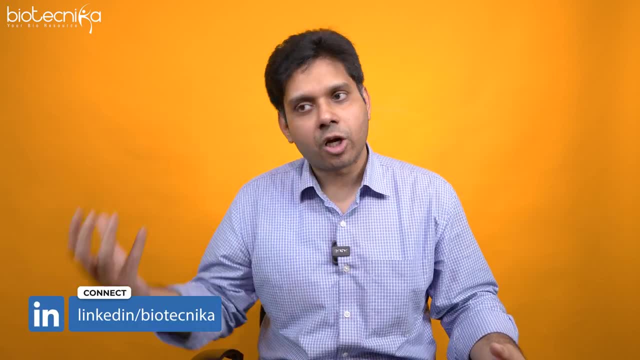 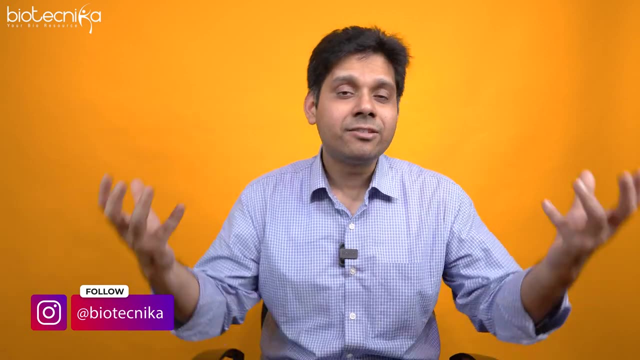 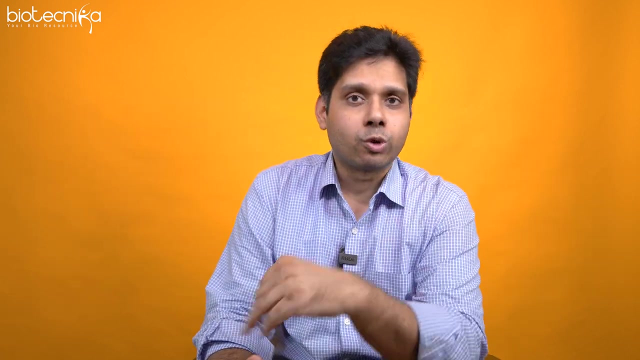 is on a biological side is predominant, while in computational biology the computers and mathematics is predominant. so that is where the uh the difference would be and that is where they both complement each other, because when you combine both, then only you will learn. so more or less you will have to learn both. okay, question to be asked. 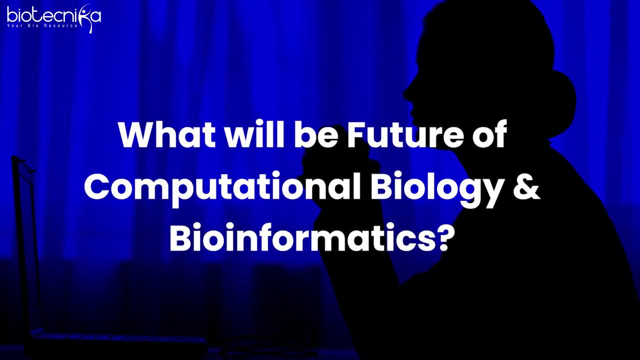 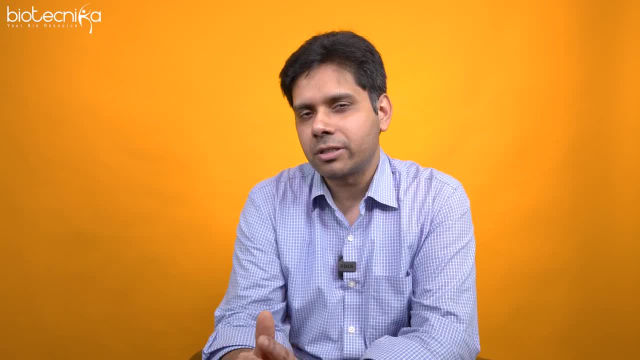 is: what will be the future of this? what will be the future of computational biology? what will be the future of bioinformatics? so i have answered this question in multiple details, in many, uh, much more detail in different videos, but just in one line: see advanced data analysis is the future. 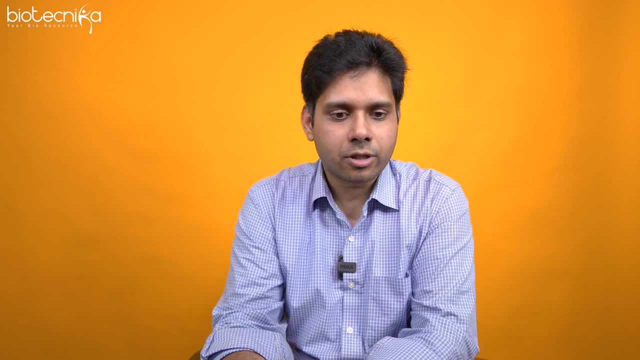 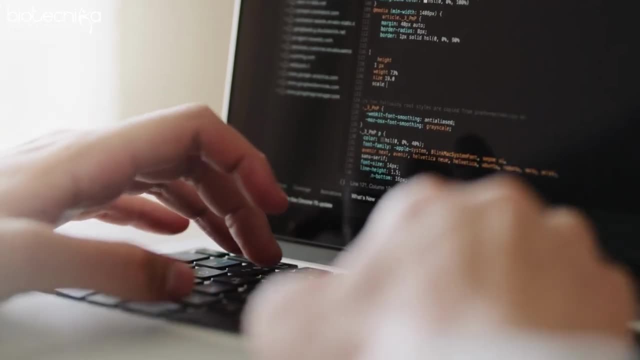 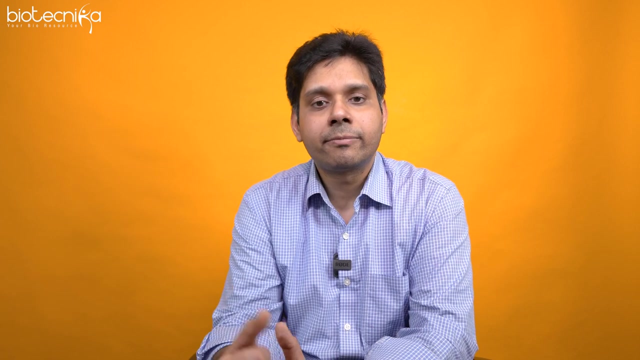 biological data is in like petabytes of storage. uh, today, and to do it? today, scientists are working on developing more sophisticated algorithms and computational methods for analyzing complex data sets in biology. the same with integration of multi-omics data set. so we combine the data from genomics, transcriptomics, proteomics, etc. etc. to gain a more comprehensive 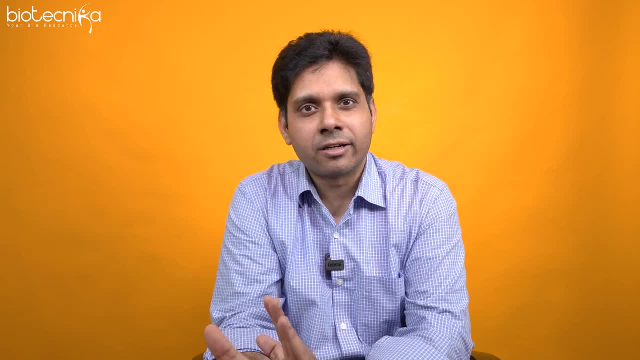 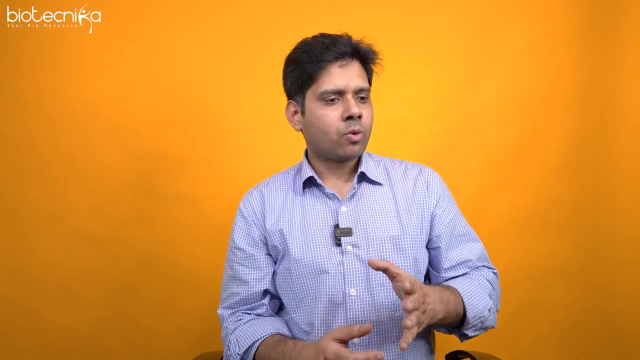 view of the biological systems. so this is more or less the difference and similarity and the future scope. now many students i'm sure will ask me: okay, so after my bachelor's in bioinformatics, can i go for a massive computational biology, or after my computational biology, can i do a phd in this? 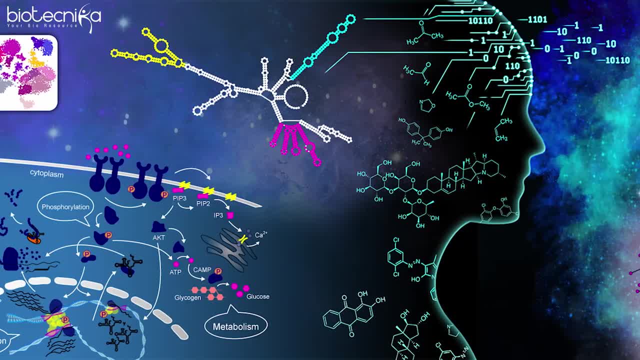 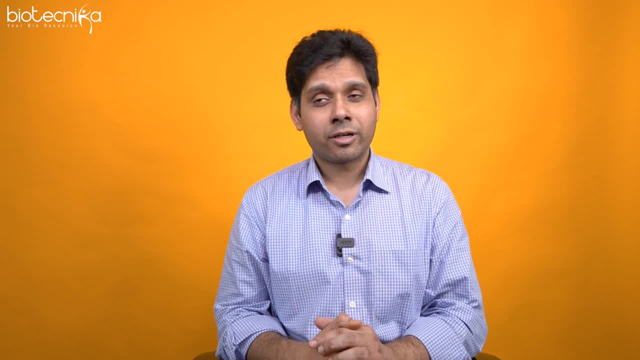 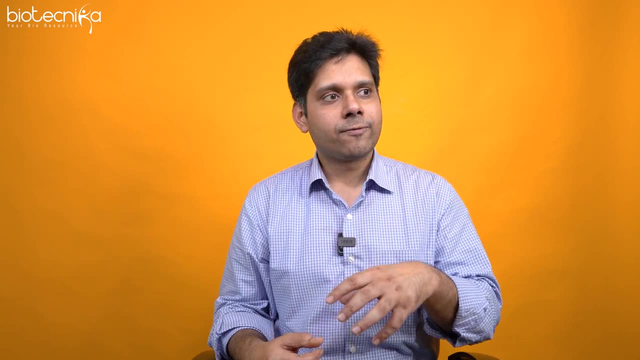 see how i see it is. computational biology would be a more advanced format. you can always do it are more or less the same. but at the end of the day, where your career grows is when you learn how to use it for commercial development. you, if you are just a academic guy who will do a 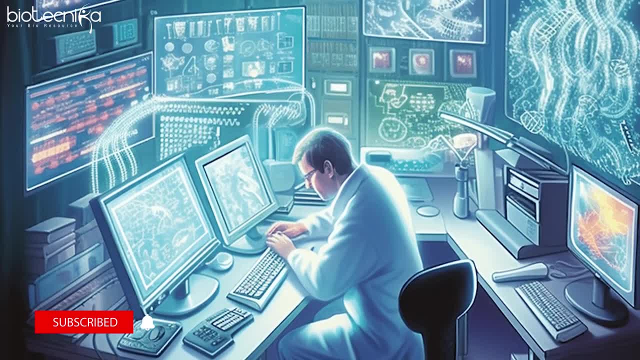 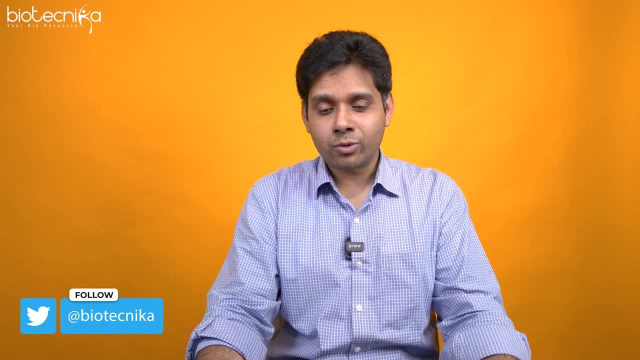 phd and just sit back, relax as a professor, then you are not going into the industry and doing challenging jobs- and i'm not saying the professors are not doing. they're doing a challenging job of teaching the students. but what you studied in applying that in a commercial establishment.